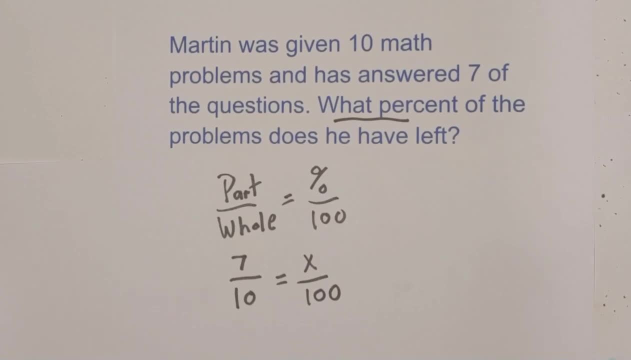 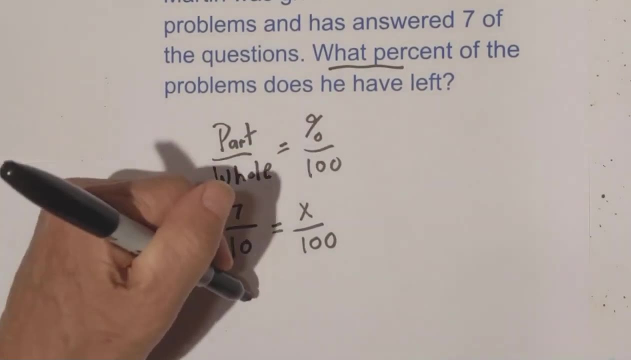 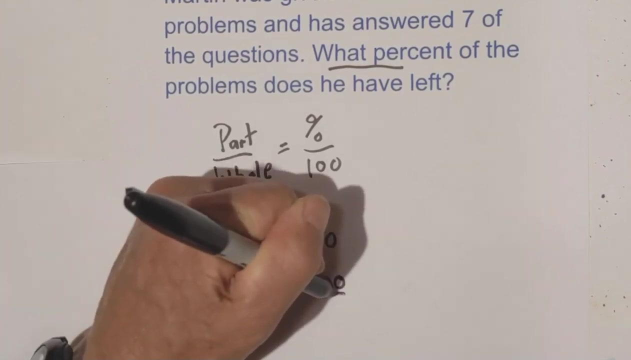 Then all you do is cross, multiply and then solve for X. I'm gonna move it up a little bit more. So X times 10 is 10. X is equal to 7 times 100 is 700.. Solve for X, Divide both sides by 10.. Bring down the X and that is 70. So 70 is 70 percent. but 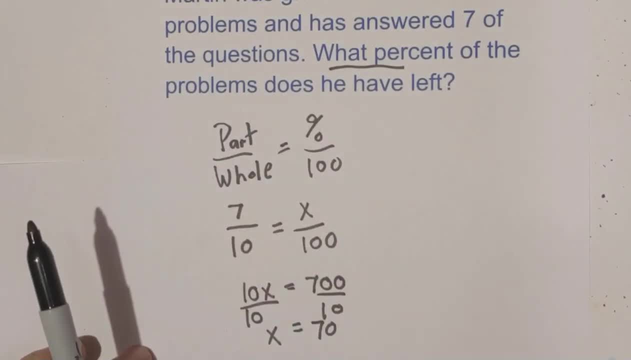 remember is: what percent does he have left? So now what we're going to do is have to do is take 100 minus 70, because that's how many he has completed, but we want to know how many he has left, and 100 minus 70 is 30. So he has 30 percent. 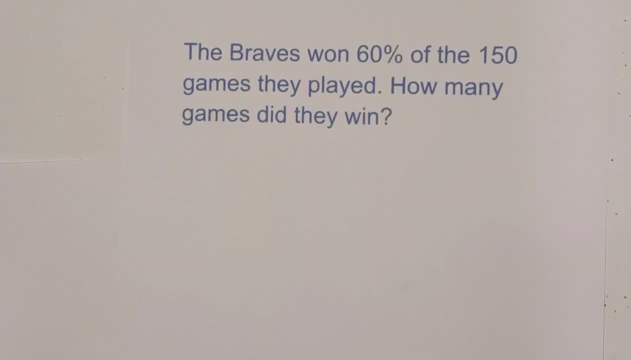 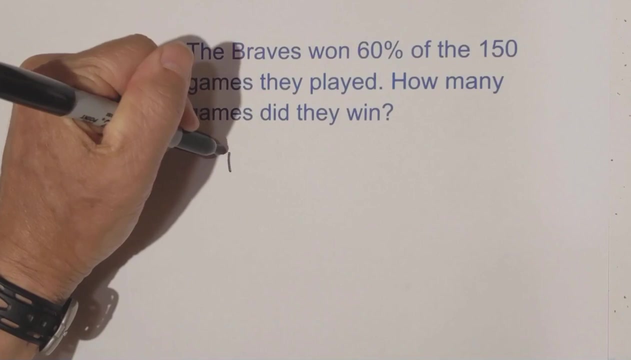 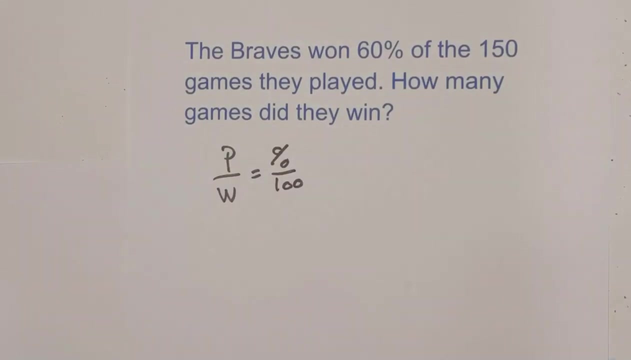 left. Let's try a couple more of these. Okay, the Braves won 60% of the 150 games they played. How many games did they win? Again, we're gonna try: part over whole equals percent over 100. And then we're just gonna see what we're given. Well, we know we're given the 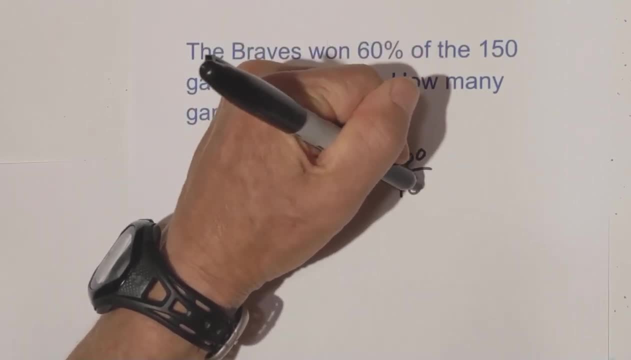 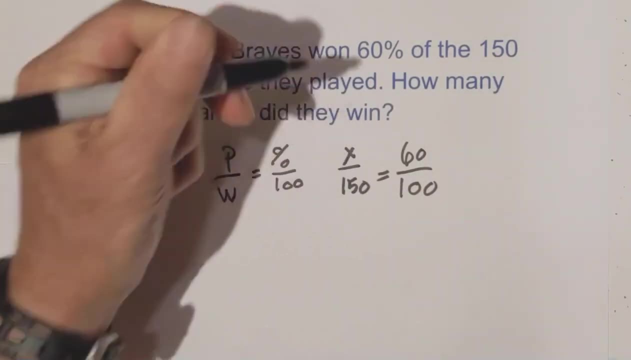 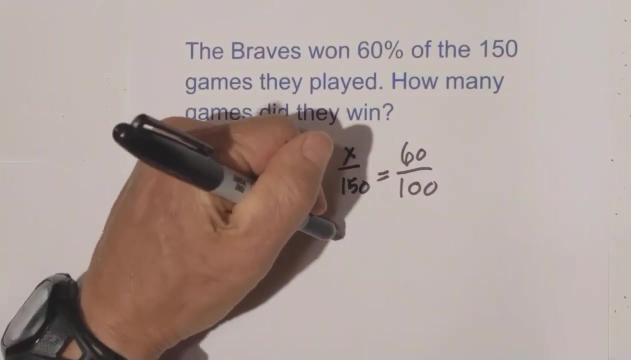 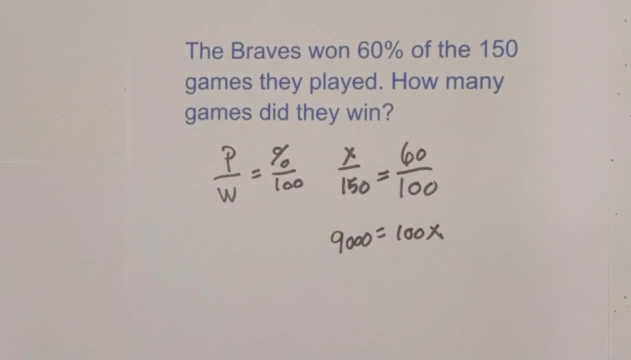 percent. so we have 60% over 100 equals and 150. that is the whole, And so we're gonna try to find X. So now all we do is we do a cross multiplication: 60 times 150 is 9000 is equal to 100 X, because X times 100 is 100 X. 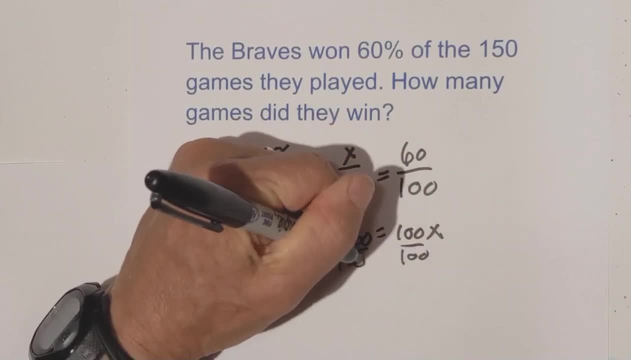 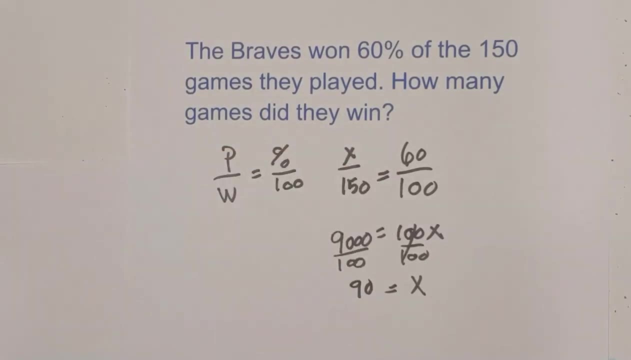 Now we divide both sides by 100. Those cancel out 9000 divided by 100 is 90. So the original question is: how many games did they won? Did they win? Excuse me, They won 90 of their 150 games, which is 60 percent. Okay, now let's take a look at. 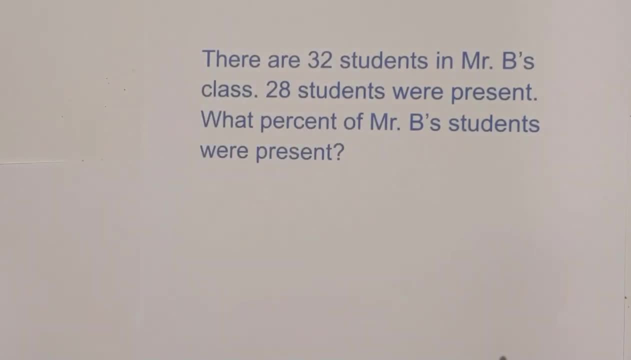 this one. There are 32 students in Mr B's class. 28 students were present. What percent of Mr B's students Were present? So here we go Again. we're gonna use part over whole, equals percent over 100.. Okay, let's see, there are 32 students, so that's gonna be the.